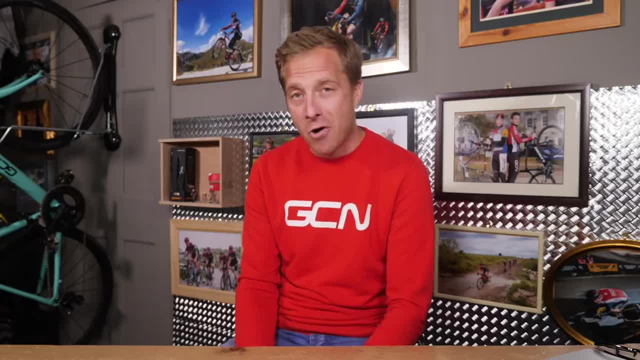 that needs some lubricant, And quite often they apply the wrong one. Few kilometers, few miles down the road, and they hear that squeaking sound or, even worse, the dry metallic noise. If you've heard it, you'll know all about it. 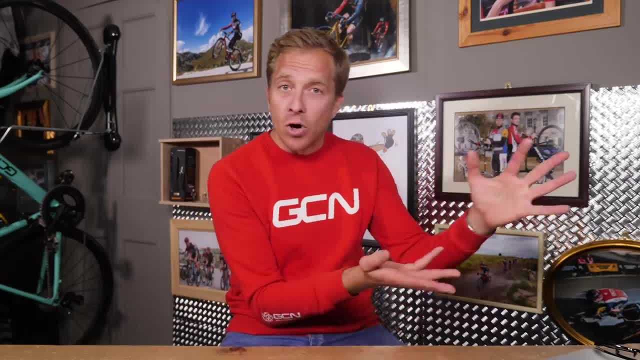 If you've heard it, you'll know all about it. If you've heard it, you'll know all about it, The reason being: it's just simply washed off. Now, in the winter months, it's vital you get the right lubricant on there. 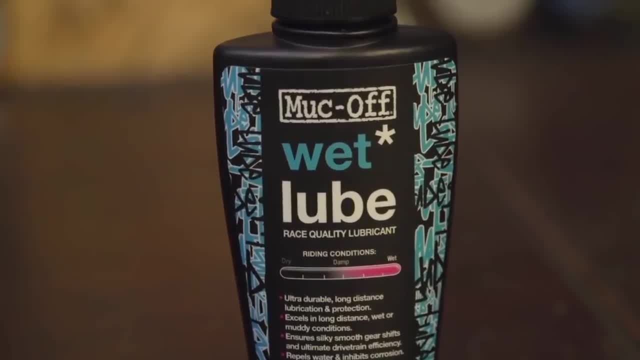 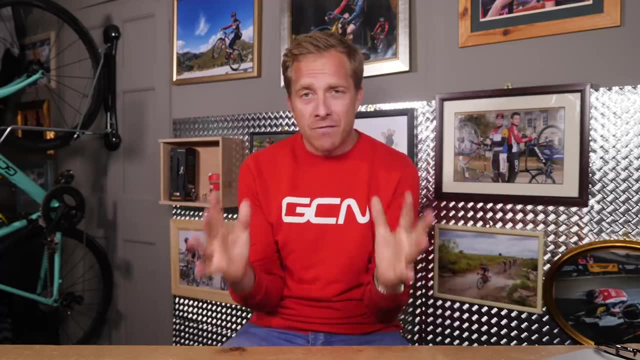 So you wanna use a wet lube, but put the right amount on. If you go and cover it well, you're gonna attract every known bit of grime, dirt, sand, road debris you can find on the road. It's gonna clog up the chain, it's gonna wear it out. 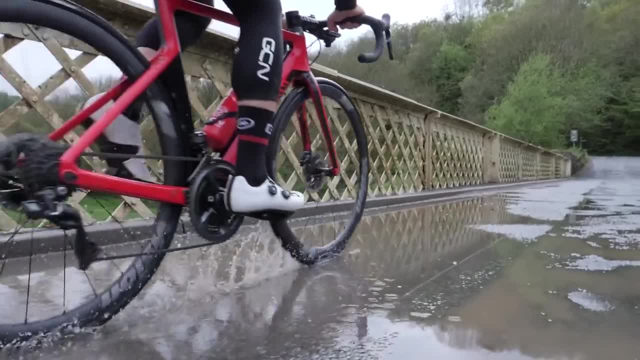 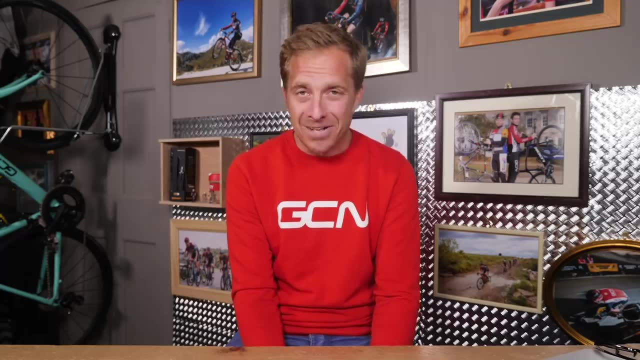 which is never good. So keep the wet lube for wet conditions, because the dry stuff is never gonna stay on the chain, And keep the dry lube for the dry conditions. It sounds logical. it is logical If you use the wet stuff in the dry. you're gonna attract all of the dirt and grime from the road to your drive train quicker than ever. It's gonna almost be like a magnet. trust me, Been there, done that, got the grubby chain. Now many of you, I'm sure, own more than one bicycle. 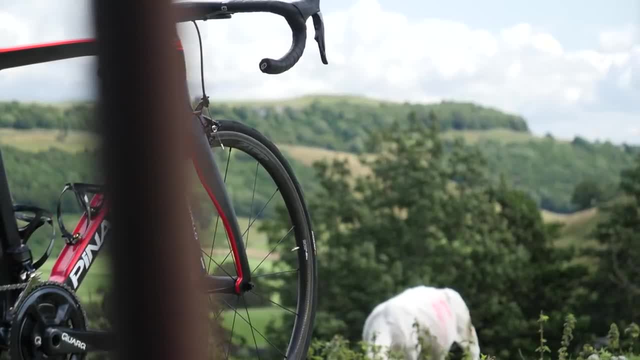 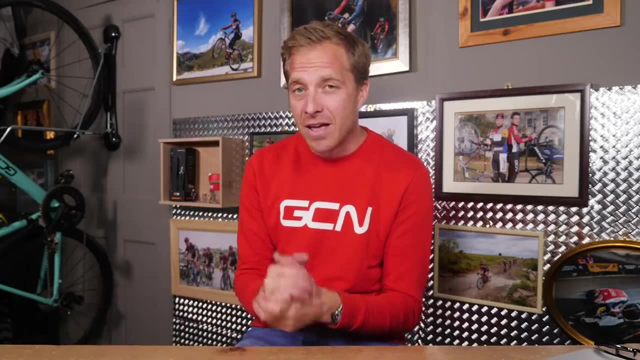 And if you've got a top of the range lightweight bike, if you use that all year round relentlessly, you're gonna end up wearing it out pretty quick, Because in the winter months, if you don't take care of it, those lightweight components aren't gonna last that long. The entry level stuff tends to be slightly harder wearing And essentially it's gonna cost you in the long run if you just wanna show off to your mates on that top of the range bike. If you've got a winter bike, make sure you use it. 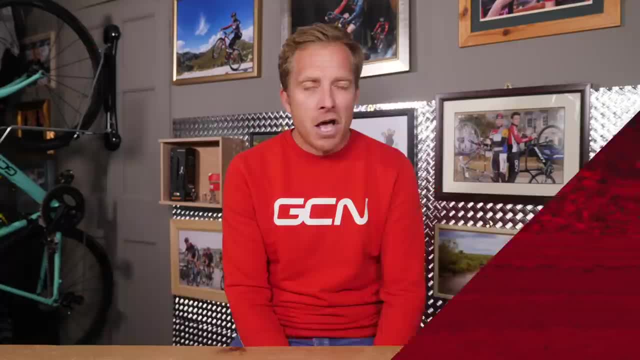 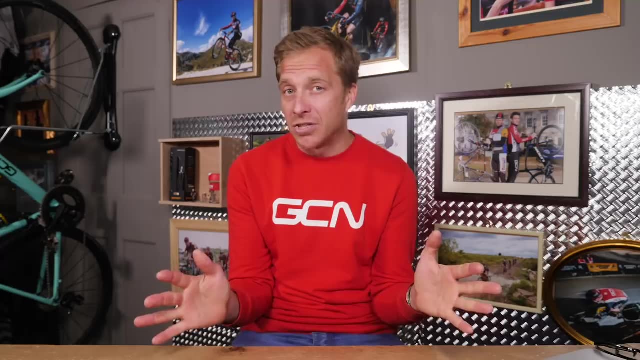 And also keep it nice and clean. Avoiding stress on parts of your bike is certainly gonna add to its lifespan. Now, it's easier said than done in some situations, particularly if you're riding in the middle of a group and someone doesn't point out a pothole. 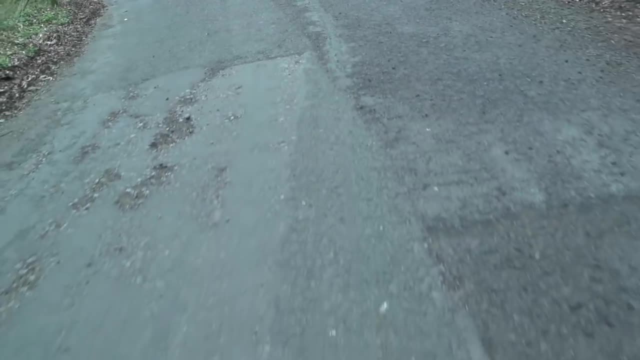 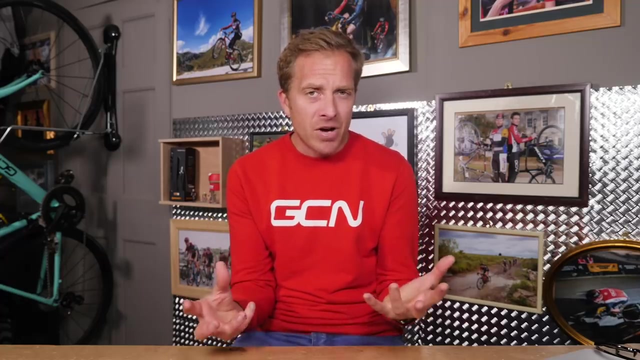 But you can almost be prepared for it, even if you don't have time to undertake a bunny hop. So one way you can do it is to kind of release a little bit of weight from the actual bike itself. Now, you are not gonna be able to do that, obviously. 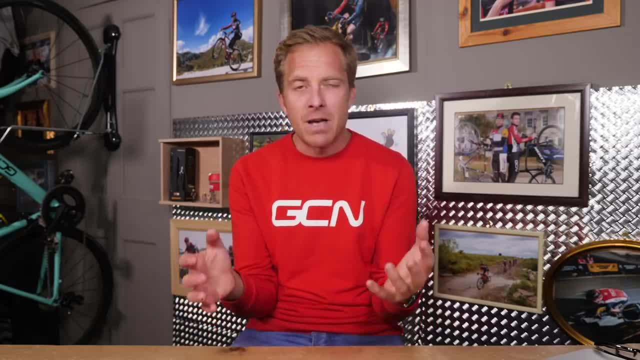 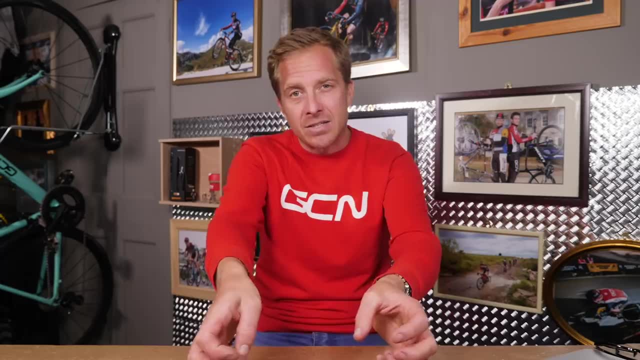 without getting off of the bike, but you could use your limbs kind of as a bit of suspension. So let your arms take a bit of the shock out if you were to ride into a pothole, so you're not forcing it inside. 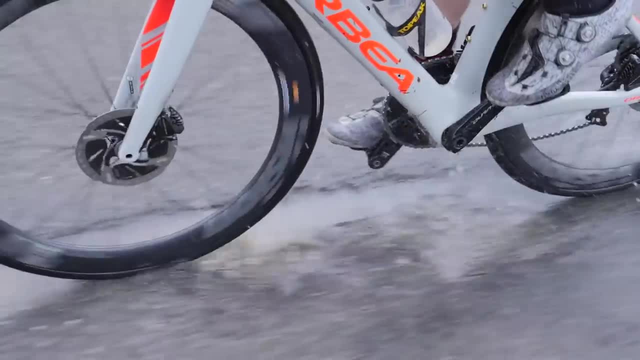 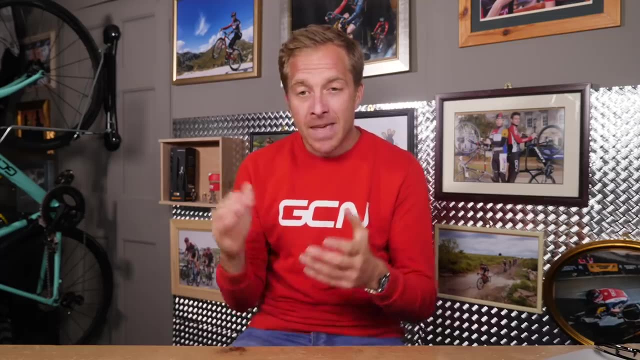 It's rather finding its own way out, And likewise with the back wheel it's gonna help you out. With the back wheel, lift your bum from the saddle and let that wheel kind of float over it or float through it a little bit easier. If you flat spot or dent that rim you're gonna know about it, and on the way home it's likely it could cause you more problems than ever, And quite often it's difficult to get hold of replacement rims. Yeah, been there, done that one too.